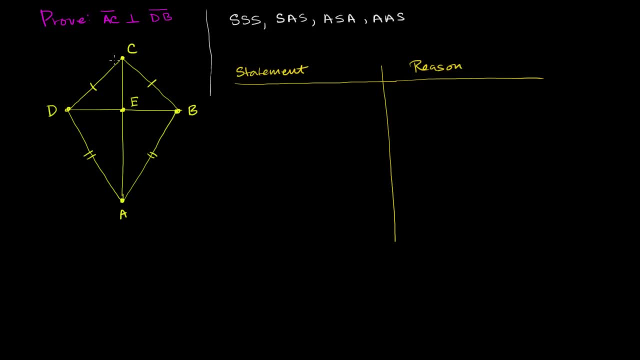 it seems like I can prove that triangle CDA is congruent to triangle CBA, based on side, side, side. And that's a pretty good starting point, Because once I can base congruency then I can start to have angles be the same. 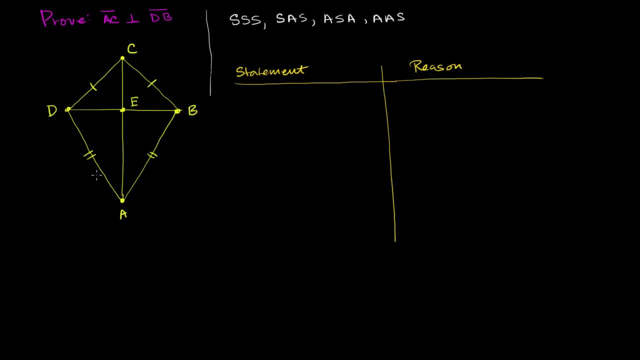 And the reason why I can do that is because this side is the same as that side, This side is the same as that side And they both share that side. But I don't want to just do it verbally this time. I want to write it out properly in this two-column proof. 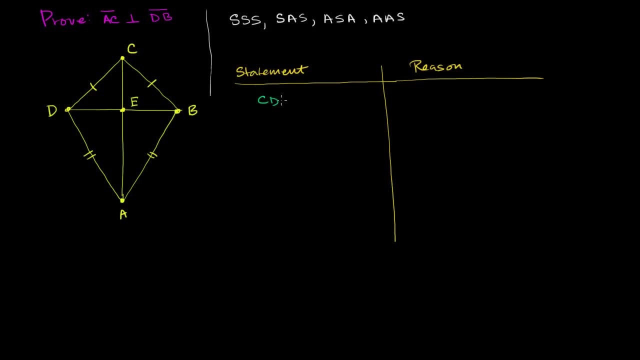 So we have CD, We had the length of segment. CD is equal to the length of CB. CD is equal to CB and that is given. That is given. So these two characters have the same length. We also know that DA the length. 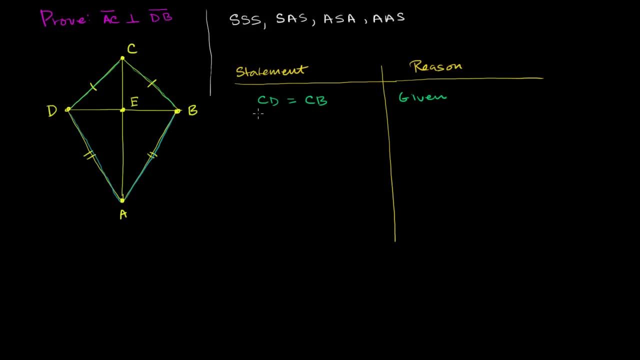 of segment DA is the same as the length of segment BA, So DA is equal to BA. That's also given in the diagram. And then we also know that CA is equal to a CA. I guess we could say So: CA is equal to itself. 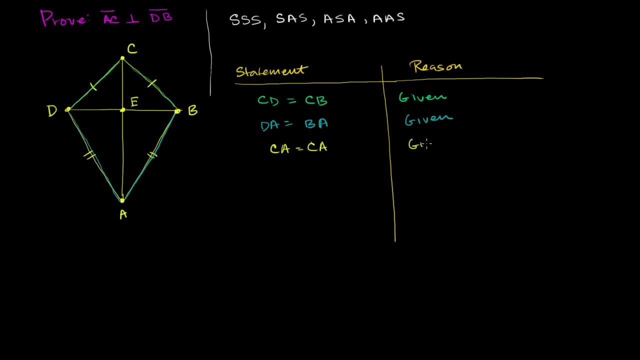 And it's obviously in both triangles. So this is also given, or it's obvious from the diagram Or obvious from the diagram. It's a bit obvious. Both triangles share, They share that side. So we have two triangles. Their corresponding sides have the same length. 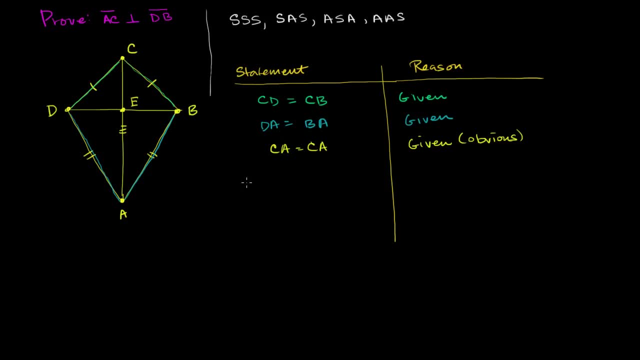 And so we know that they are congruent. So we know that triangle CDA is congruent to triangle CBA And we know that by the side, side, side postulate and the statements given up here. Actually, let me number our statements just. 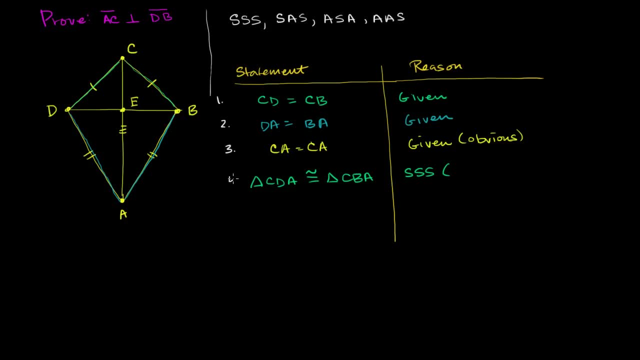 so we can refer back. Let's go back to this: 1,, 2,, 3, and 4.. And so side side side postulate, and 1,, 2, and 3.. Statements 1,, 2, and 3.. 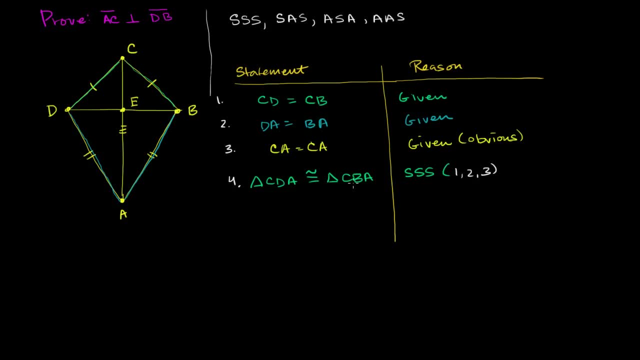 So statements 1,, 2, and 3 in the side side postulate: let us know that these two triangles are congruent And then, if these are congruent, then we know, for example, we know that all of their corresponding angles 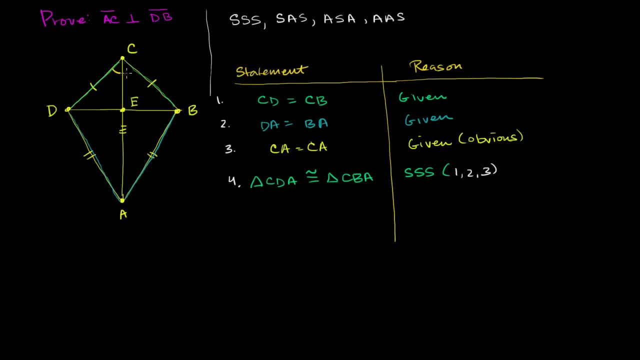 are equivalent. So, for example, this angle is going to be equal to That angle. So let's make that statement right over there. We know that angle DCE, So this is going to be statement 5.. We know that angle DCE. that's this angle right over here. 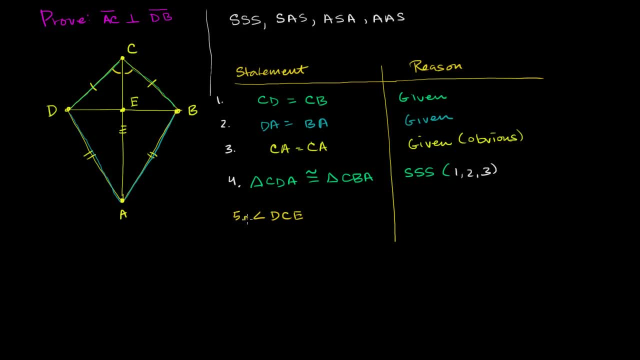 is going to have the same measure. We can even say they're congruent. I'll say the measure of angle DCE is going to be equal to the measure of angle of BCE, And this comes straight out of statement 4.. This comes straight out of statement 4, congruency. 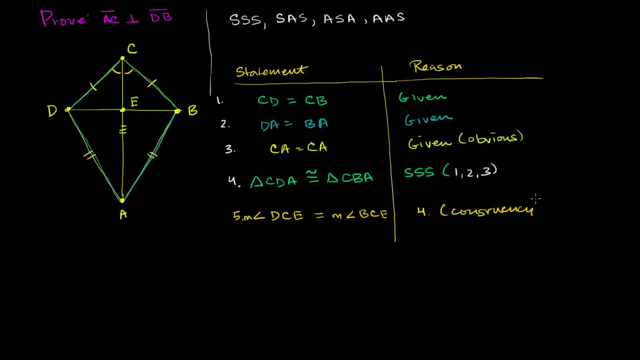 OK, I could put in parentheses Congruency of those triangles. This implies straight, because they're both part of this larger triangle. They are the corresponding angles, So they are going to have the exact same measure. Now it seems like we can do something pretty interesting. 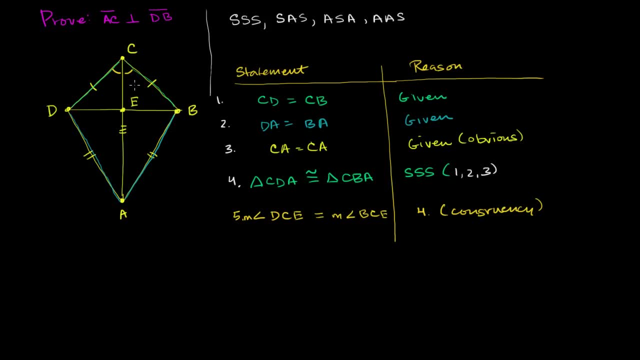 with these two smaller triangles at the top left and the top right of this looks like a kite-like figure, Because we have a side. Two corresponding sides are congruent, Two corresponding angles are congruent And they have a side in common. They have this side in common right over here. 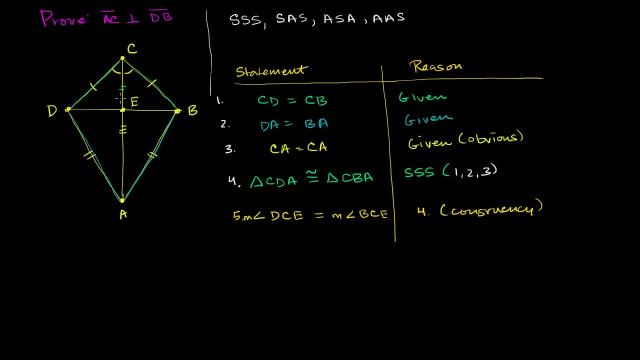 So let's first just establish that they have this side in common right over here. So I'll just write statement 6.. We have CE. The measure or the length of that line is equal to itself. Once again, this is just obvious. 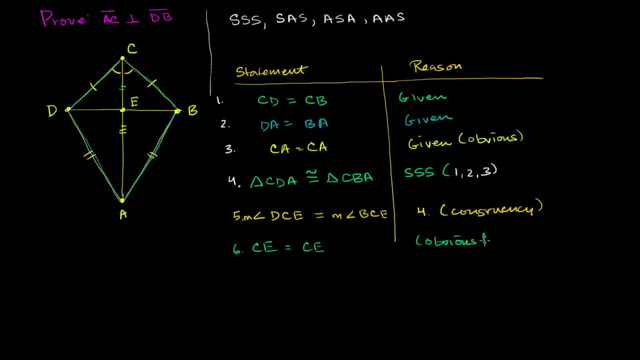 It's the same, obvious from diagram. It's the same line, Obvious from diagram. But now we can use that information. So we don't have three sides. We haven't proven to ourselves that this side is the same as this side. 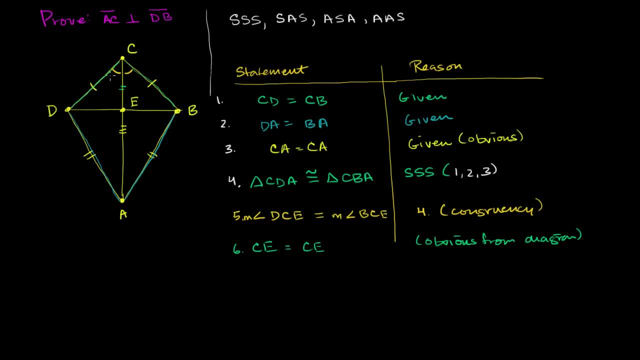 That DE has the same length as EB, But we do have a side, an angle between the sides, and then another side, And so this looks pretty interesting for our side angle side postulate. And so we can say, by the side, angle side postulate. 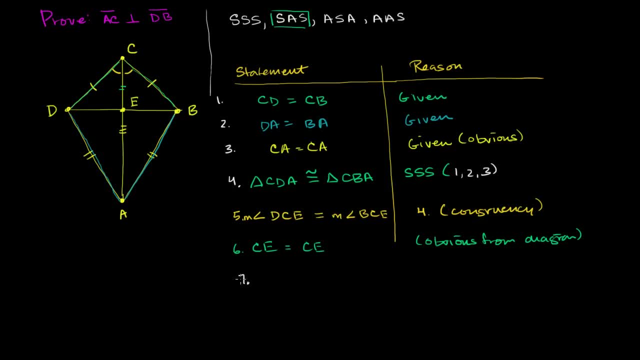 we can say that triangle DCE is congruent to triangle BCE. And when I write the labels for the triangles I'm making sure that I'm kind of putting the corresponding points. So I started at D, then went to C, then to E. 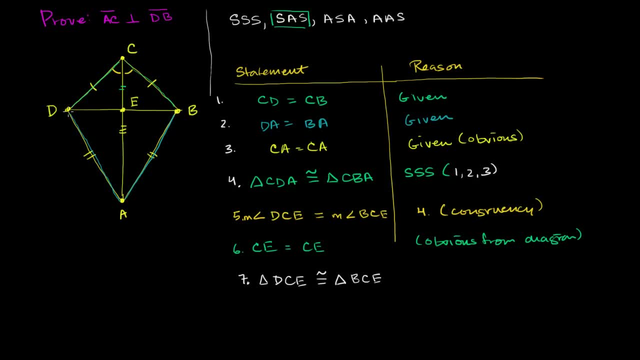 So the corresponding, I guess, angle or the corresponding point or vertex, I could say for this triangle right over here is B. So if I start with D, I start with B, C in the middle is the corresponding vertex for either of these triangles. 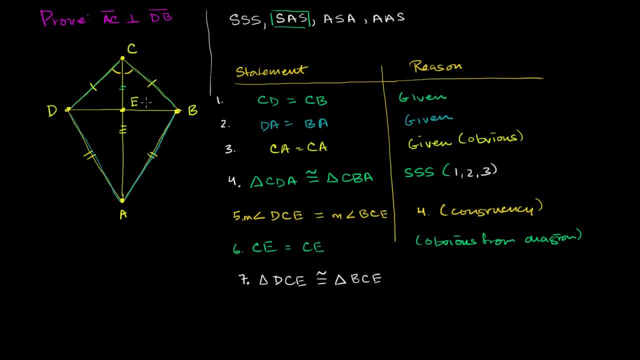 So I put it in the middle And then they both go to E And that's just to make sure that we are specifying what's corresponding to what. And we know this is true by side, angle side And the information we got from this side. 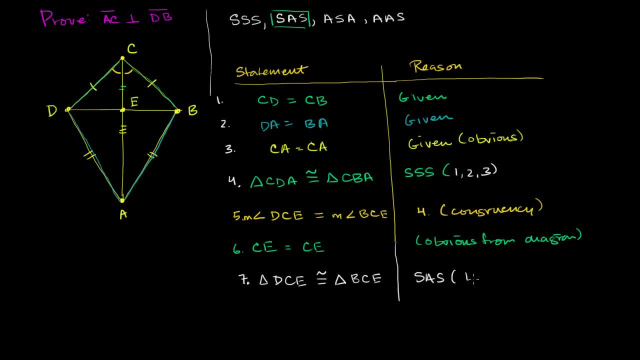 is established that these two sides are congruent was from statement one. Then that these angles are congruent is from statement five, right over here, And then statement six gave us the other side, Statement six, just like that, And if we know that these triangles are congruent, 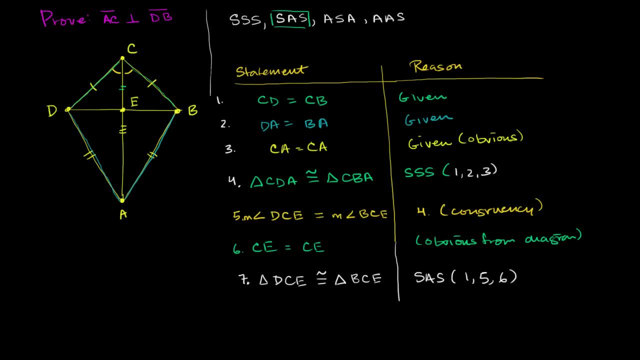 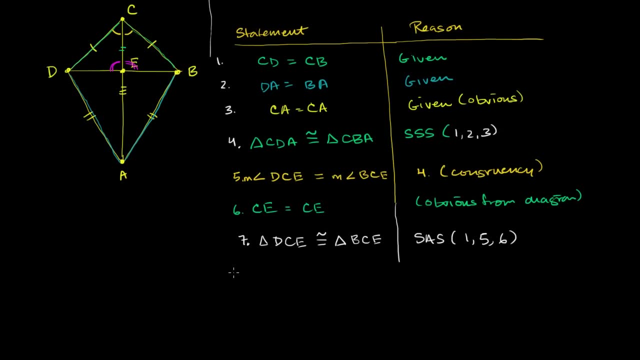 that means that all of their corresponding angles are congruent. So we know, for example, that this angle right over here is going to be congruent to that angle over there. So let's write that down, So we know. statement number eight: 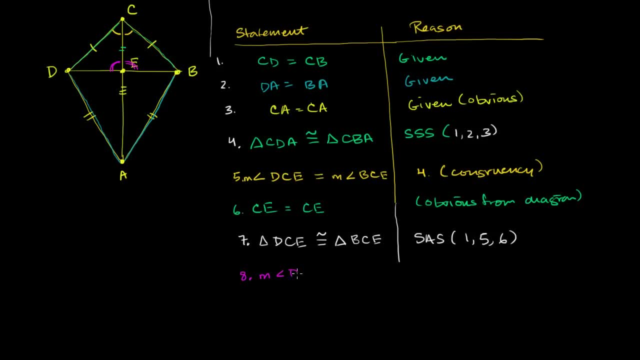 The measure of angle- let's call that DEC- is equal to the measure of angle BEC, And this comes straight from statement seven. Once again, they're congruent. And then we also know- we'll make statement nine- We also know that the measure of angle DEC. 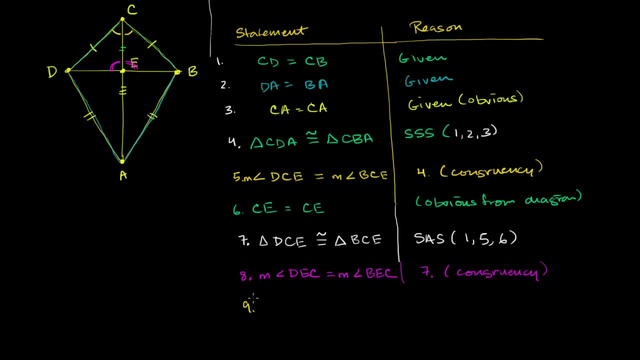 or maybe we should just write it this way: angle DEC and angle BEC are supplementary. They are supplementary And you can just look at that from inspection. But I'll write a decent are supplementary, Which means they add up their measures, add up to 180 degrees. 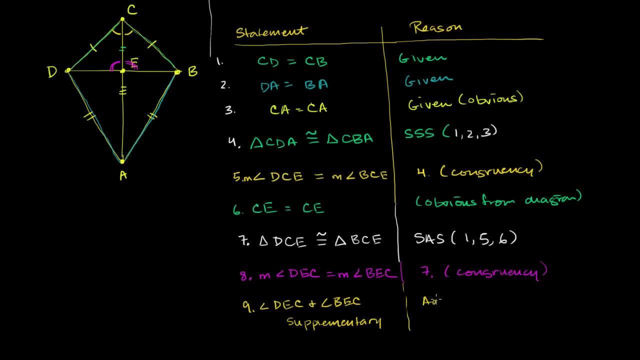 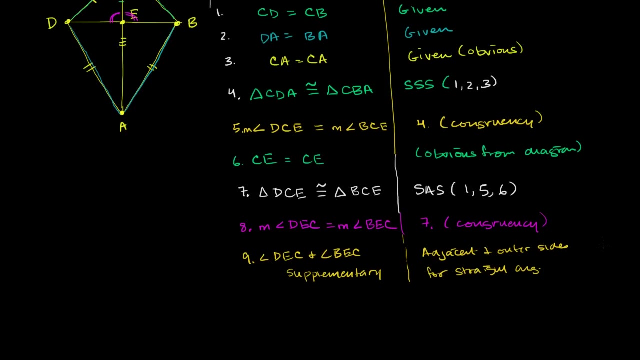 And we know that because they are adjacent, They're adjacent And outer sides form straight angle, Form straight angle, Straight angle, Straight angle. And then we can essentially the next step, if we know that these two angles are equal to each other. 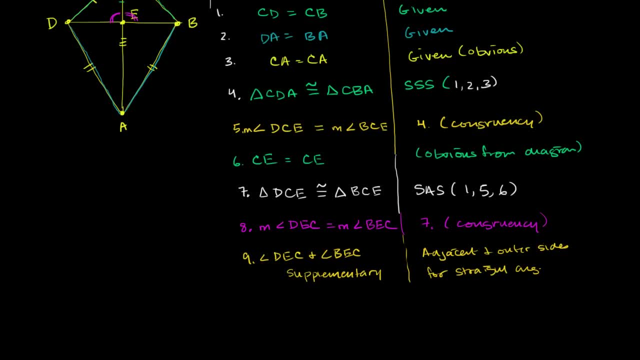 and if we know that they are complementary, our next step means that we can actually deduce that they must be 90 degrees. So 10, measure of angle DEC equals measure of angle BEC, which equals 90 degrees, And then, for the reason it might be a little bit more involved, 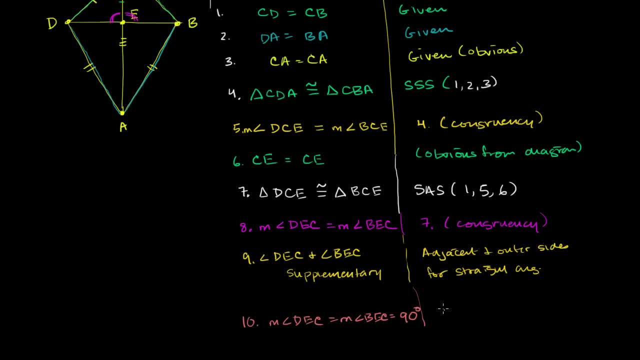 we could put these two statements together, So it would be statements eight and nine, And then statements eight and nine mean that DEC, so I could write this: measure of angle, DEC plus measure of angle of angle. Actually, let me just, since I don't want to do too many steps all at once, 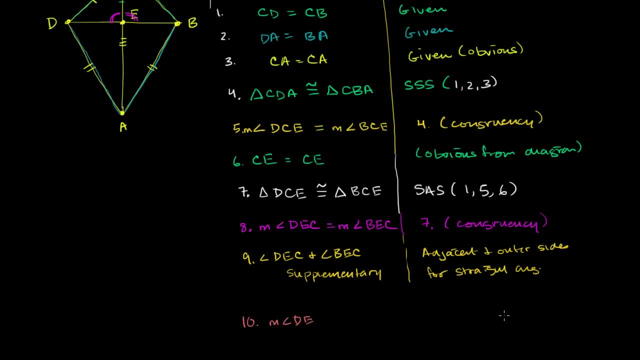 let me just take it little bit by little bit. So let me just do it all like this. So let me say measure of angle DEC plus measure of angle BEC is equal to 180.. And this comes straight from 0.9, that they are supplementary. 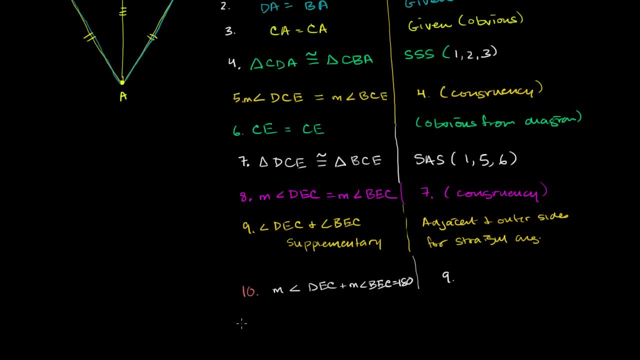 And then we could say: statement I'm done, I'm taking up a lot of space. now, Statement 11, we could say: measure of angle DEC plus measure of angle DEC is equal to 180 degrees, And we know that from statement nine and statement eight. 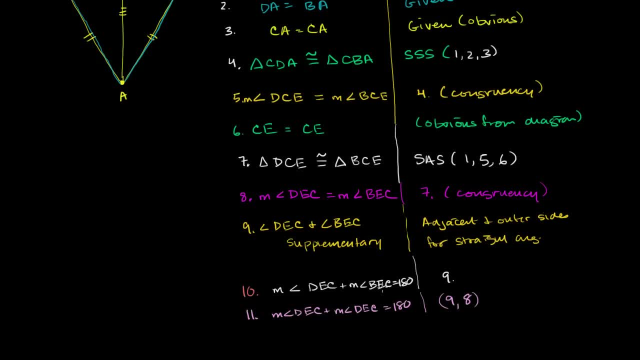 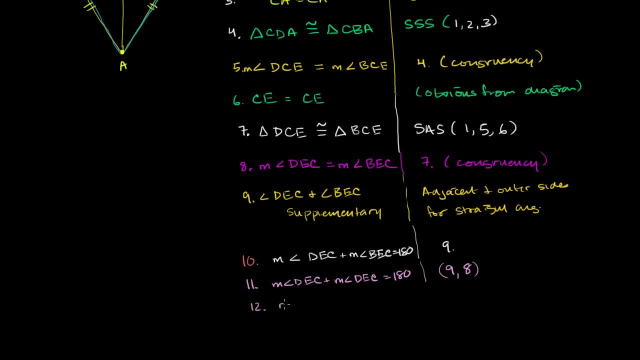 We essentially just took statement nine and substituted that BEC. the measure of BEC is the same as the measure of DEC, And so then, if we want statement 12, we could say: measure of angle DEC is equal to 90, which. 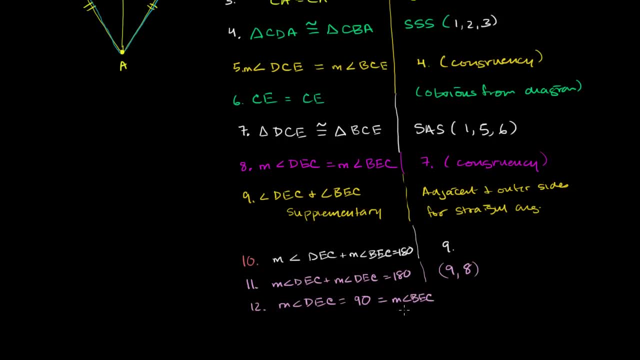 is equal to the measure of angle BEC. measure of angle BEC. And then this comes once again straight out of point number 11 and eight And what you can see, I'm kind of taking a little bit more time. 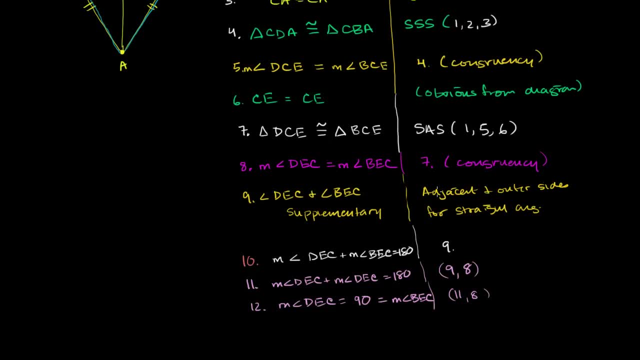 going a little bit more granular through the steps And some of the other proofs, I would have just said: oh, obviously this implies this or that, And then we're done, because if these are 90 degrees, so let me write the last statement. 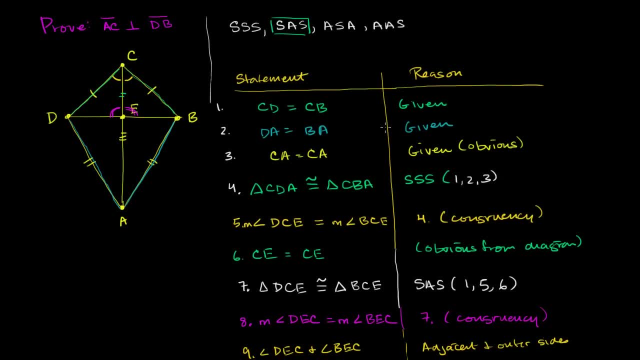 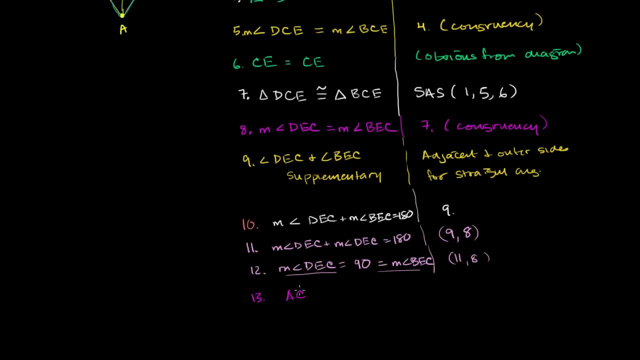 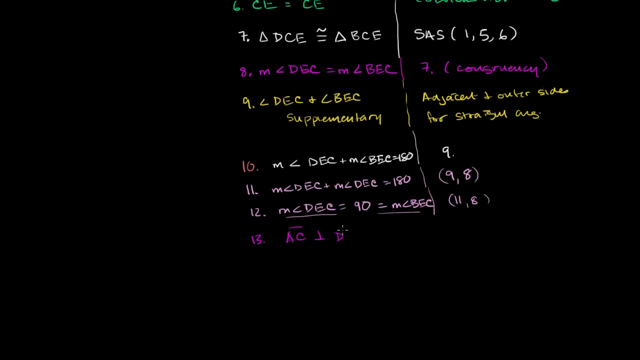 So statement 13, which is what we wanted to prove. We wanted to prove that AC is perpendicular to DB. AC is perpendicular to DB. So AC is perpendicular to what was it to? AC is perpendicular to DB, to segment DB.